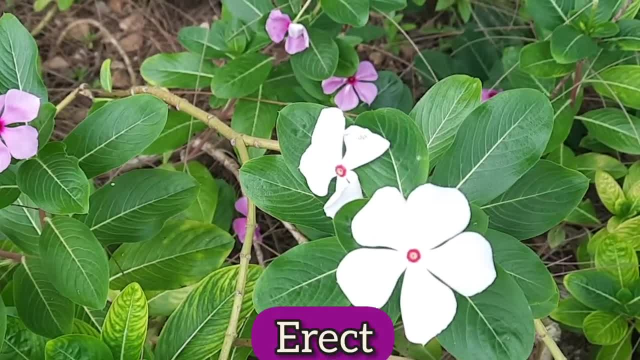 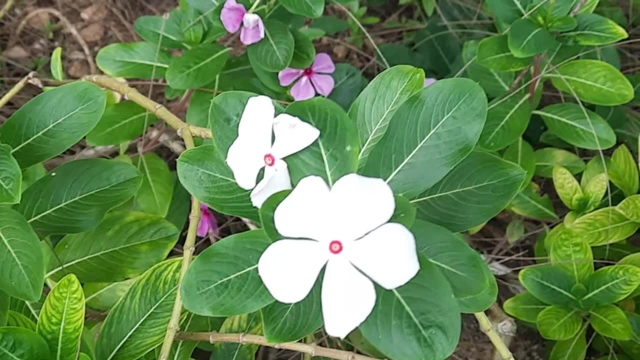 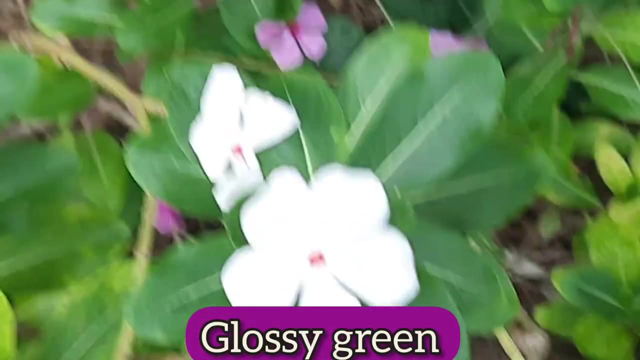 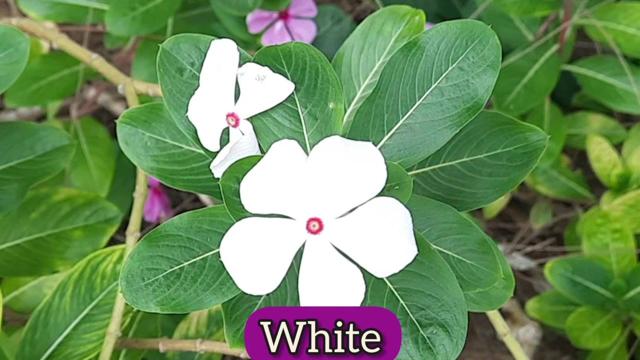 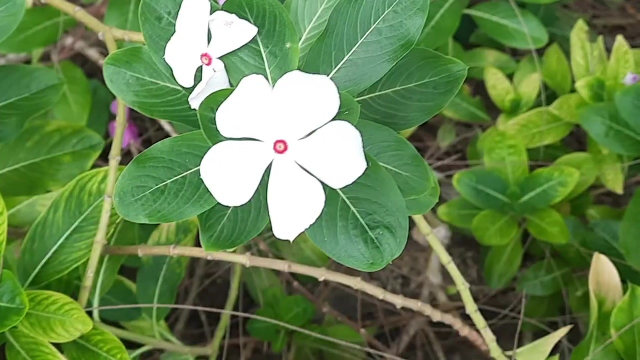 herbaceous plant. it is erect and it has branched stems that can become woody. it tends to grow between one to four feet tall. um the leaves are glossy green and the flowers have five petals and they can be pink, white or purple, and they have a purple eye in the center. the stems of the plant also produce a milky sap. 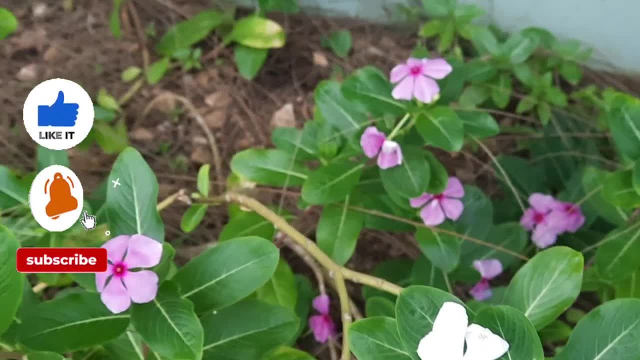 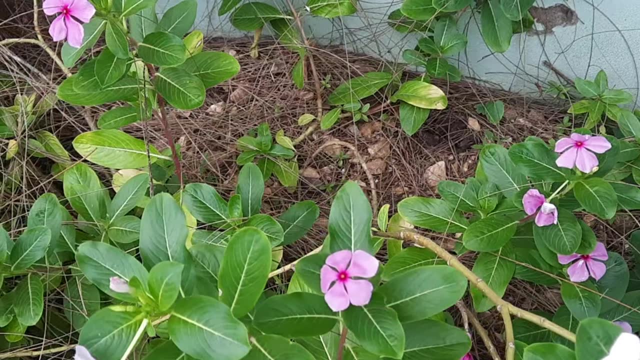 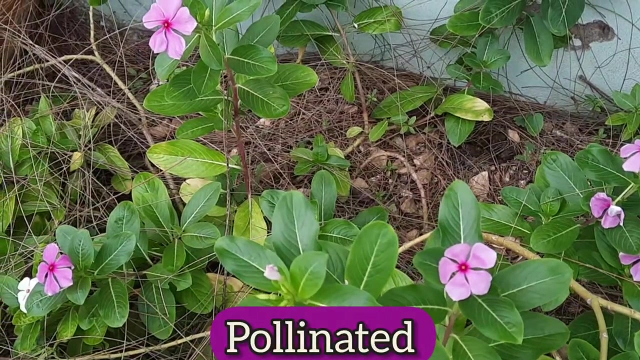 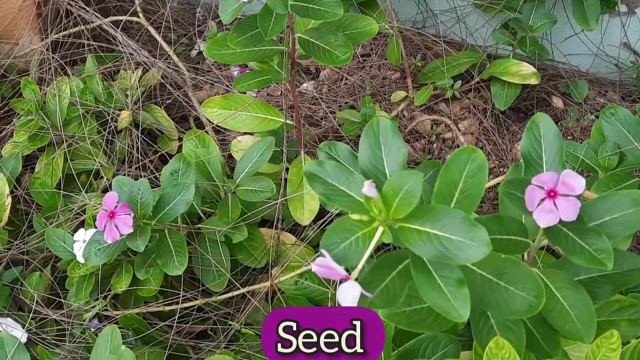 in jamaica you can pretty much find periwinkle growing in people's backyards, front yards, along roadsides and in other green spaces. the flowers are pollinated by butterflies and other pollinators, and it is usually propagated by seed or by cuttings. 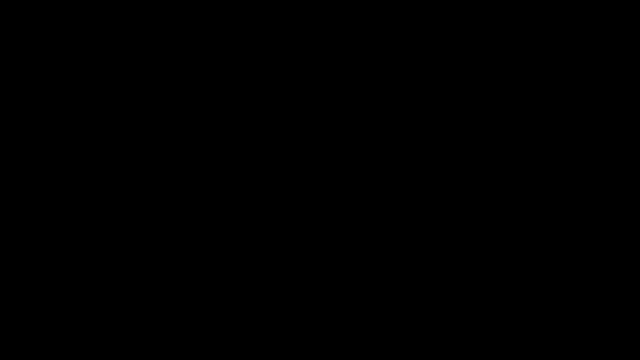 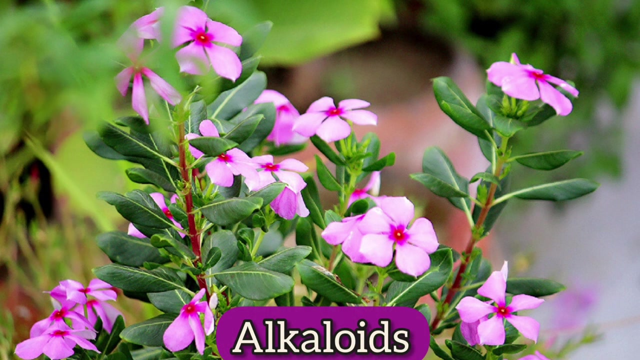 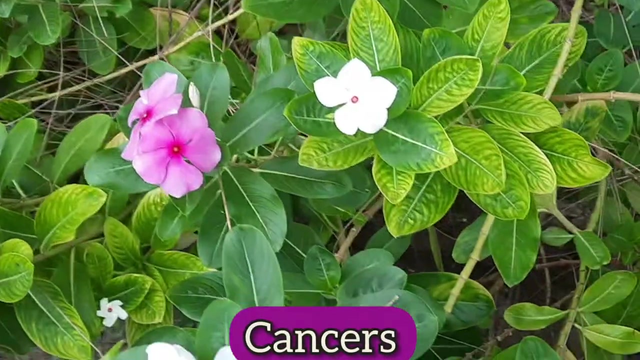 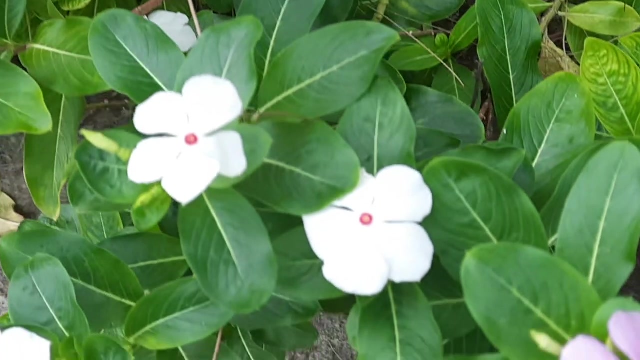 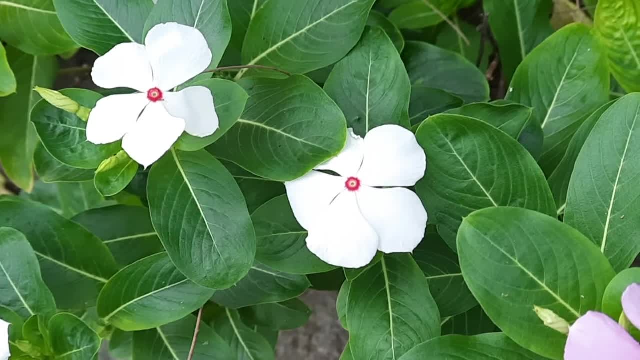 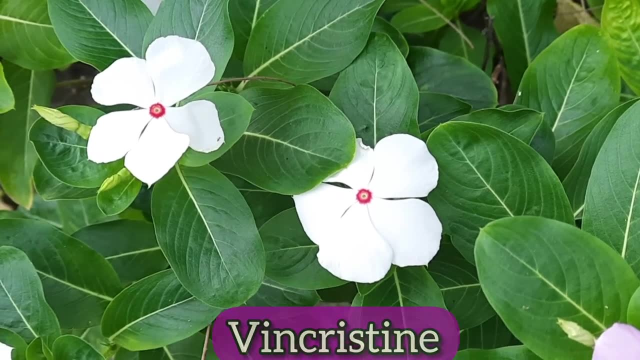 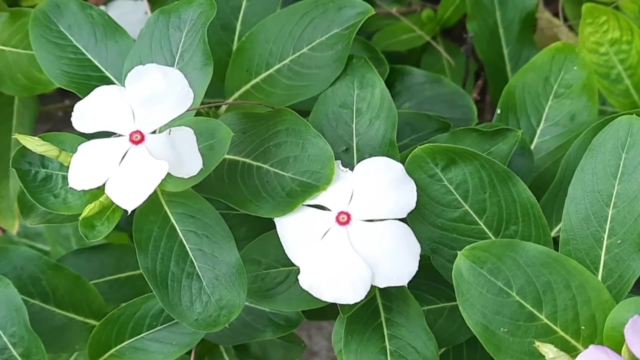 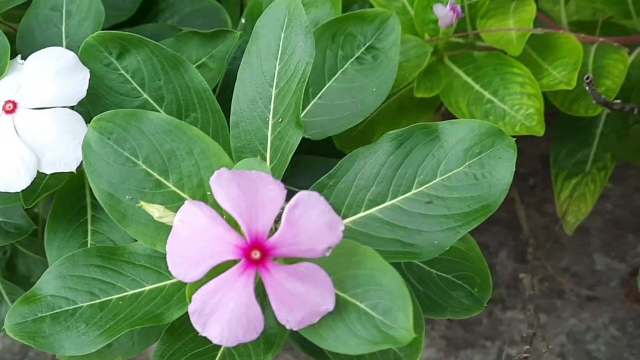 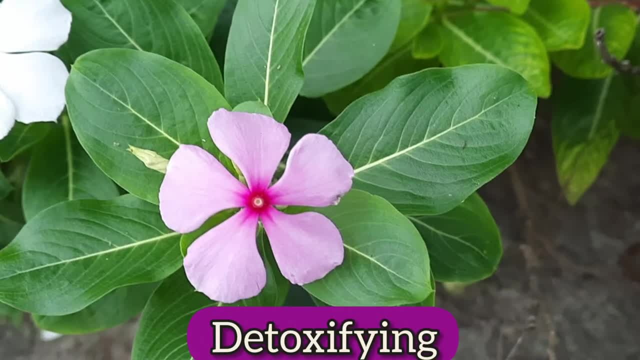 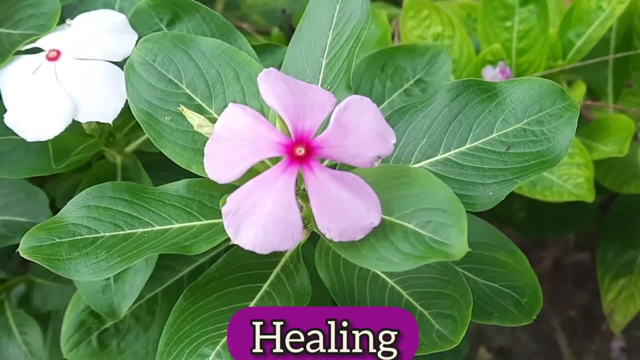 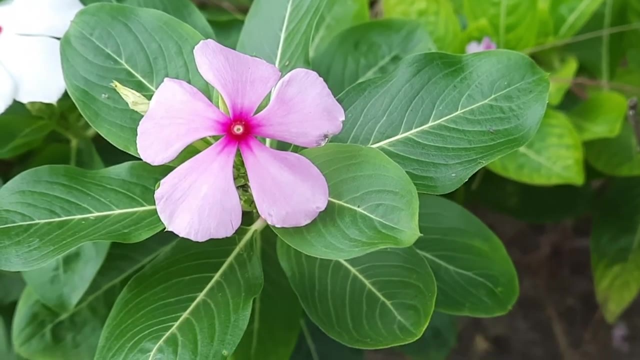 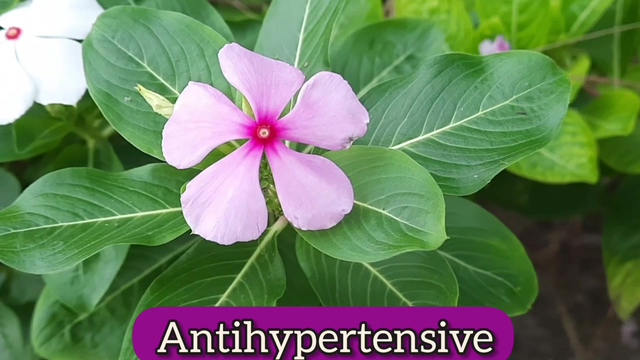 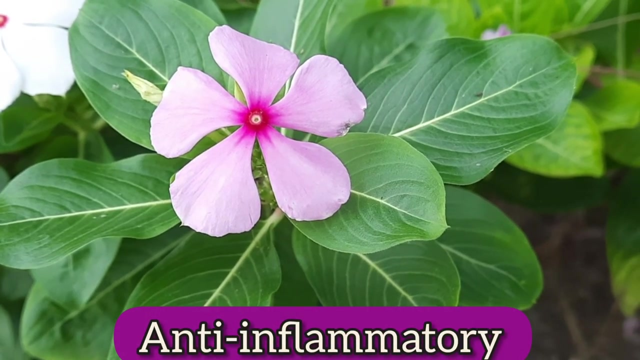 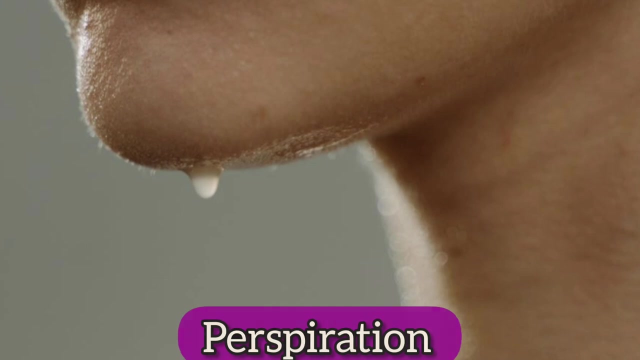 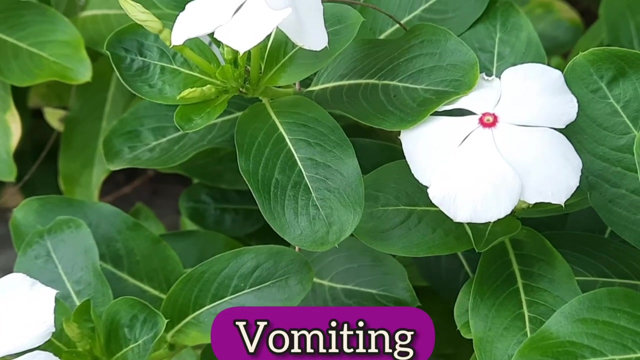 purifying, detoxifying, antimicrobial and healing properties. it also has antiviral, anti-dysenteric, anti-hyper glycemic, anti-hypertensive, anti-fertility, um and anti-inflammatory properties- um and anti-inflammatory properties. it also has properties that can increase perspiration, increase urination, promote vomiting and the boil movement, and it is also a 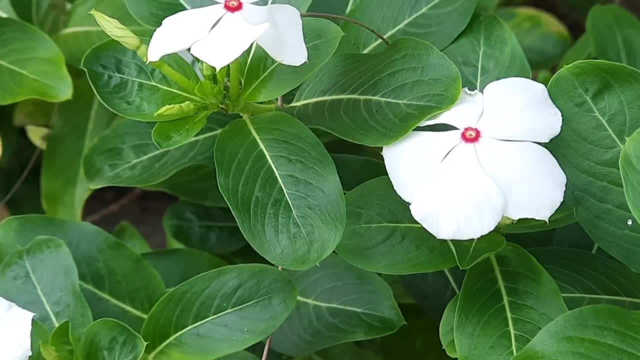 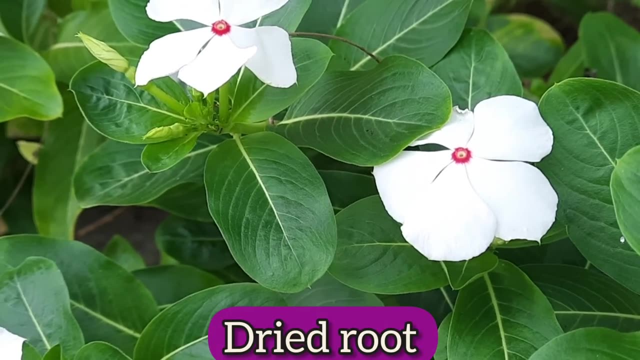 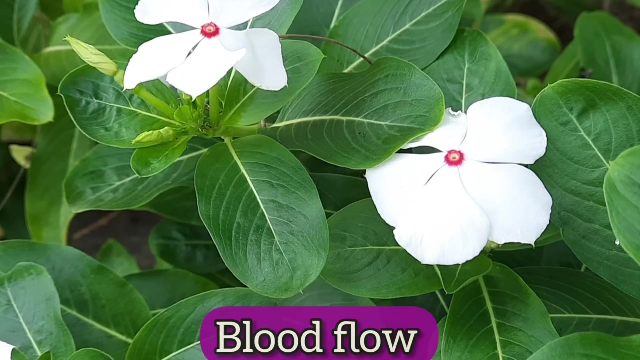 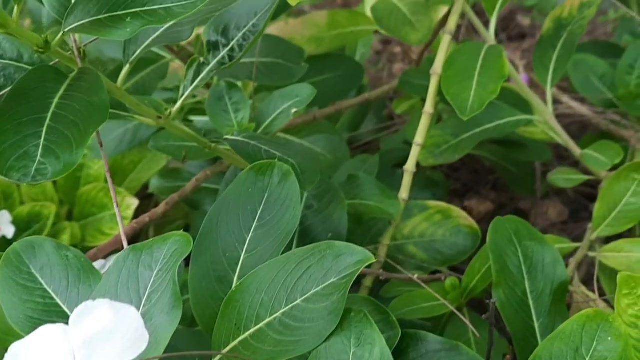 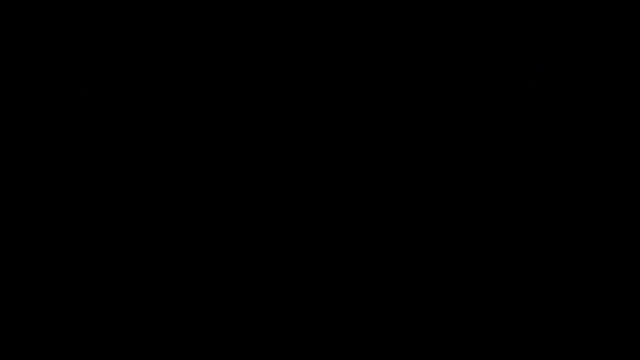 vermifuge, meaning that it has properties that can destroy or expel worms. the dried root is a source of ajmalicin, which is an alkaloid that can increase blood flow in the brain and other parts of the body. before we go any further, guys, I'm going to ask you, please, to hit that like. 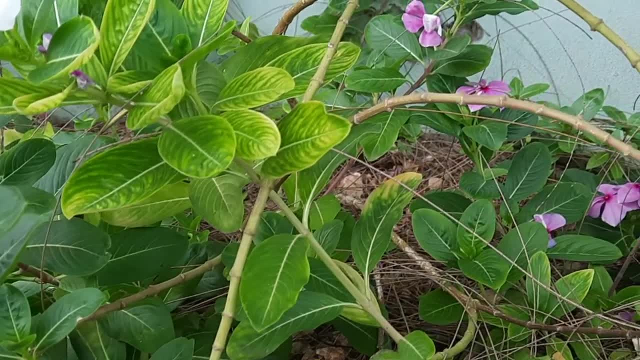 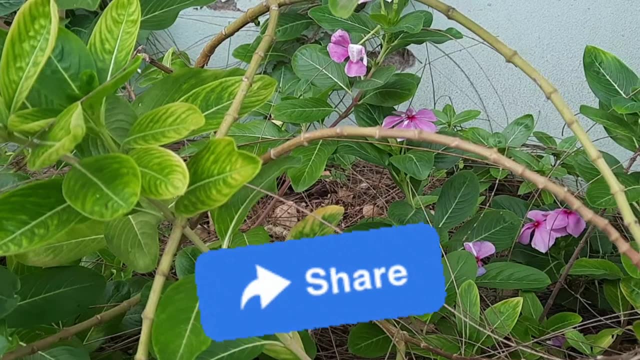 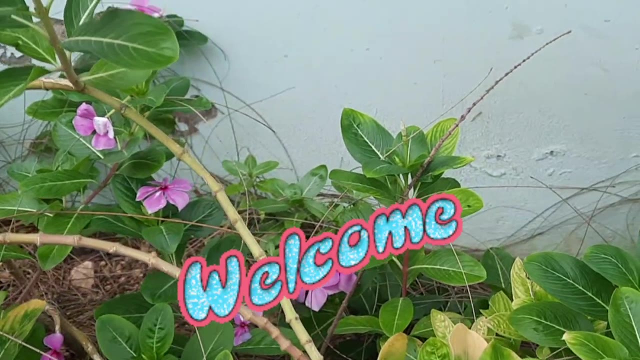 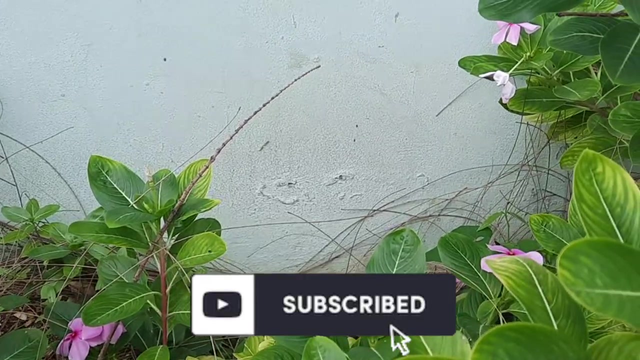 button, drop a comment and share this video as well, so that others can benefit from this information. If you're new here, a very warm welcome to you. If you would like to see more content like this one in the future, then please subscribe to the channel right now and turn that notification bell from red. 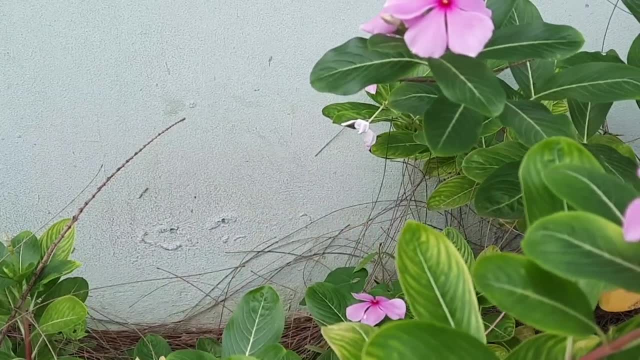 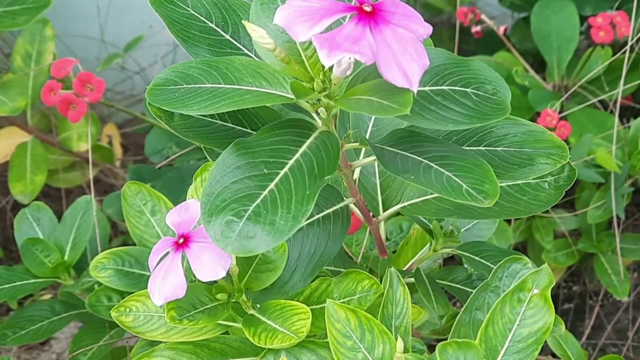 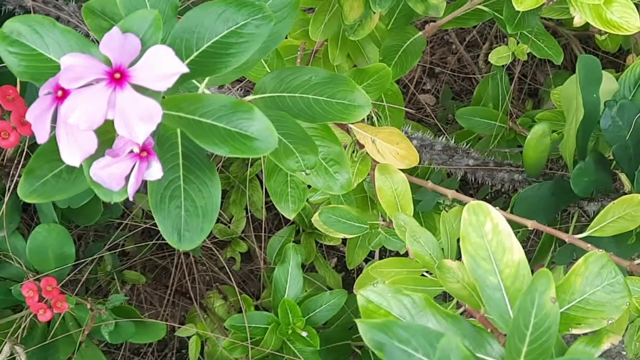 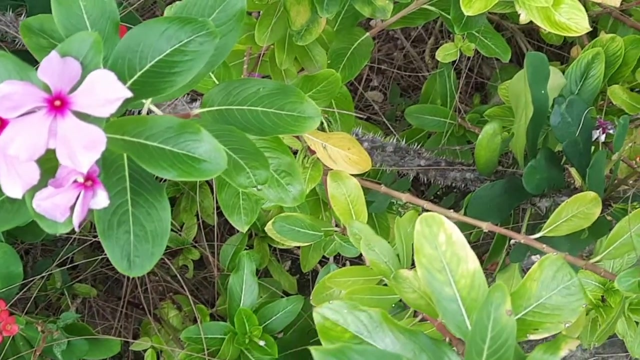 to blue, to grey, so that you won't miss our next upload. thank you so much, guys. now let's get right back to the video. so, guys, the parts of the plants that are typically used in traditional medicine include the leaves, the stems, the flowers and the. 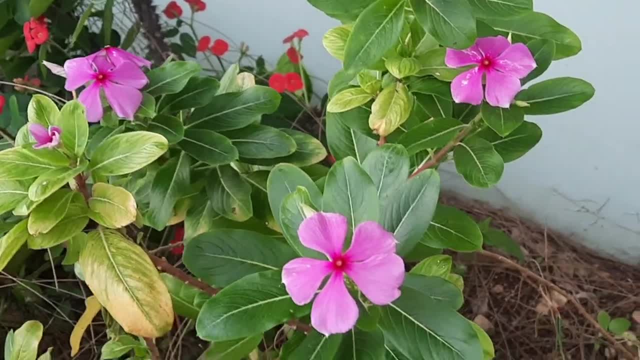 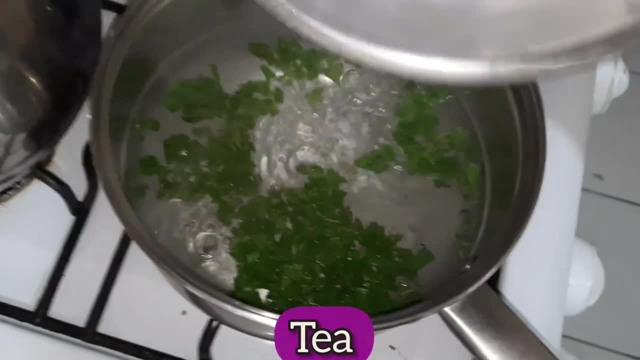 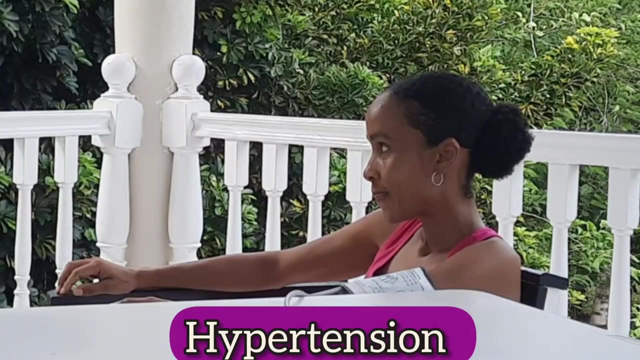 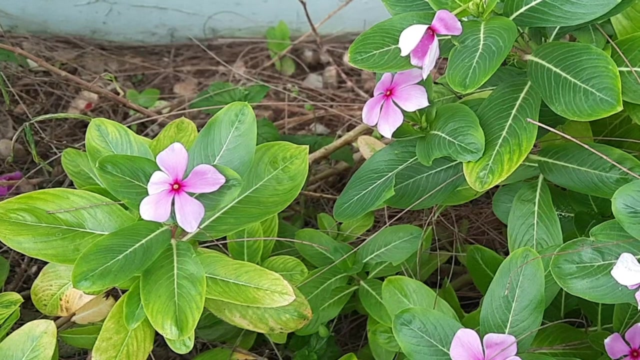 roots. in Jamaica, it is traditional for some persons to use a plant to make tea, and then they just drink this to help them to control diabetes and hypertension. this is also done in other parts of the world as well. some people use a plant to help treat various kinds of cancers. 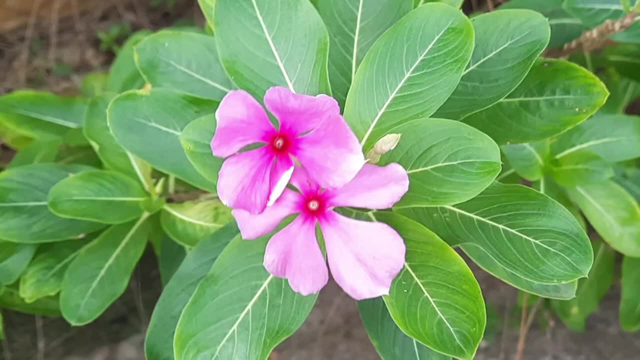 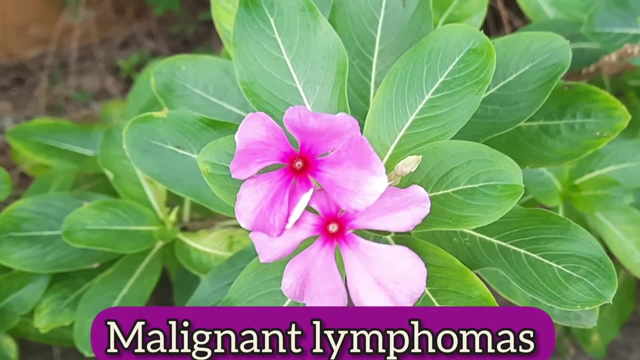 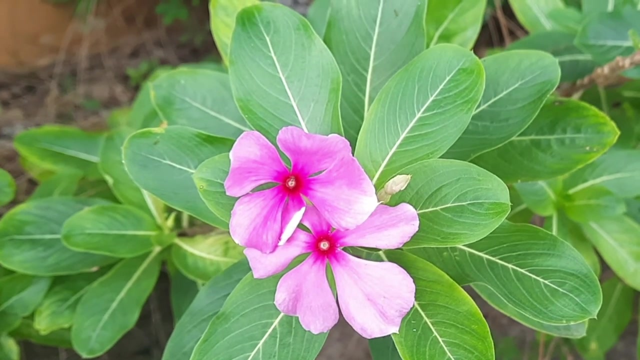 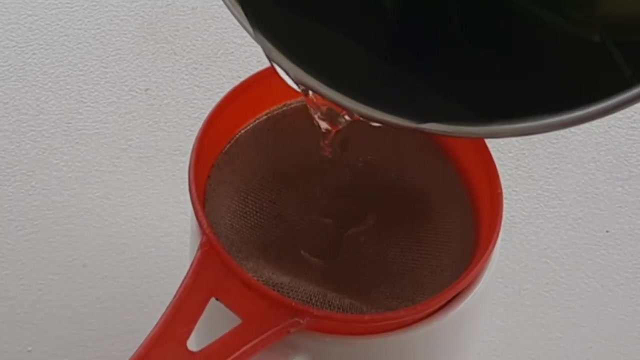 andagenies. it's done in amazing treatment of root causes of Mayor's cancer, For example breast cancer, leukemia, Hodgkin's disease, malignant lymphomas, Wilm's tumor, among other kinds of cancers. Some people also use the leaves of the plant to make tea and they take this internally to help to reduce anxiety. 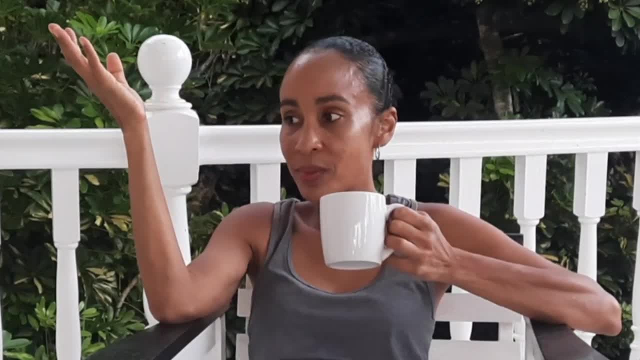 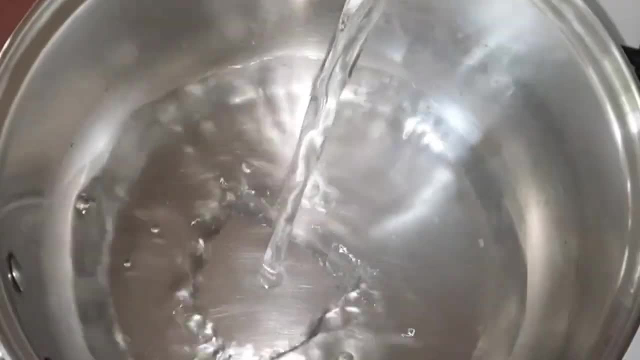 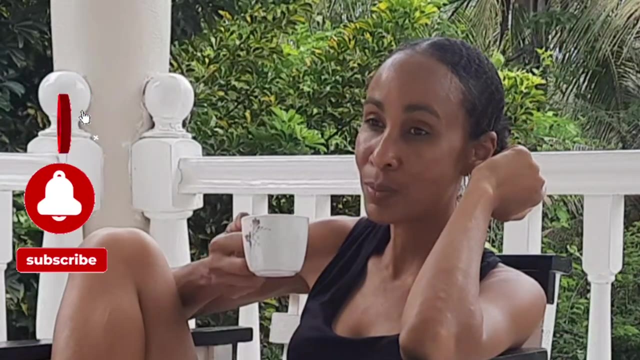 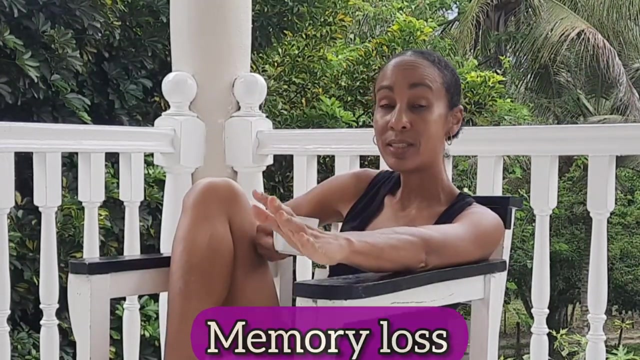 And stress, to promote sleep and to improve circulation of the blood. People also use both the leaves and stems of the plant to make tea, and they take this internally to help to treat a lot of different ailments, For example, memory loss and mental impairment that is caused from diseases like 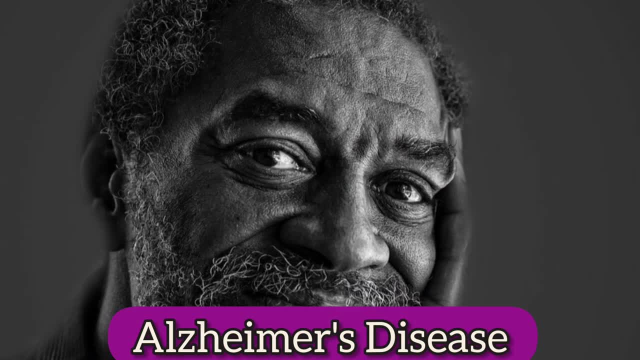 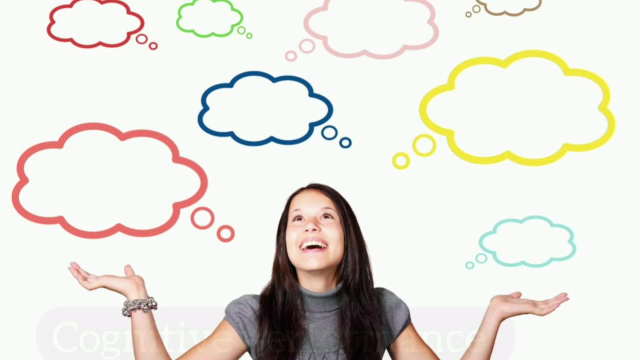 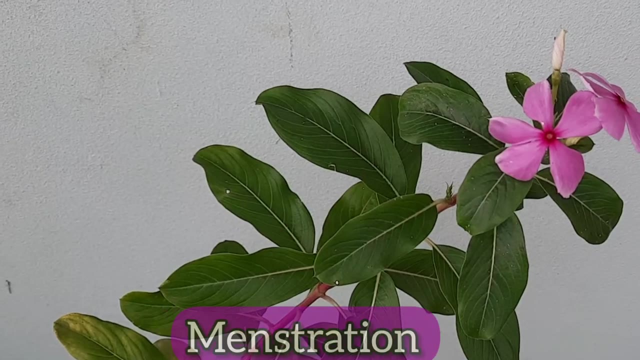 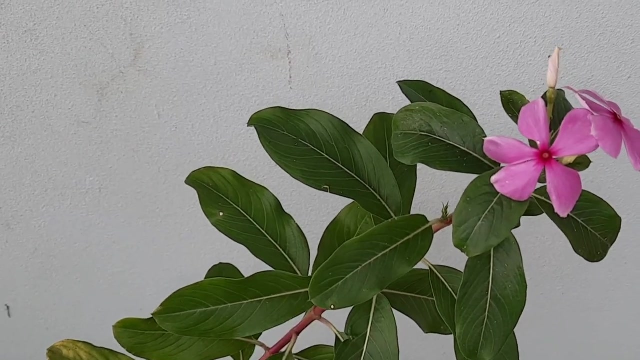 dementia and Alzheimer's disease. They also use it to promote alertness and to maintain cognitive performance, To treat headaches, irregular menstruation to help to trim down plaque in the blood vessels, To prevent a stroke and to help persons recover from a stroke. 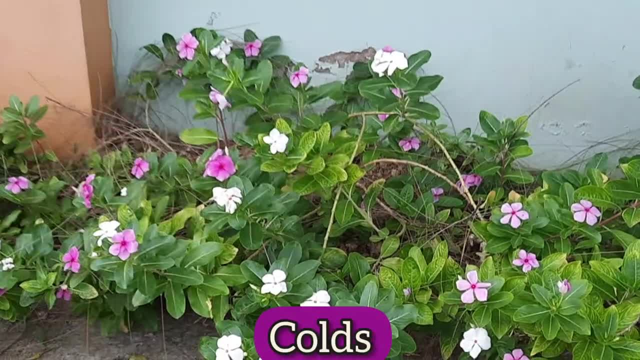 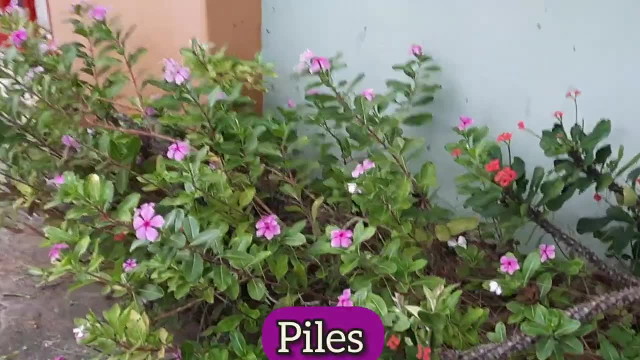 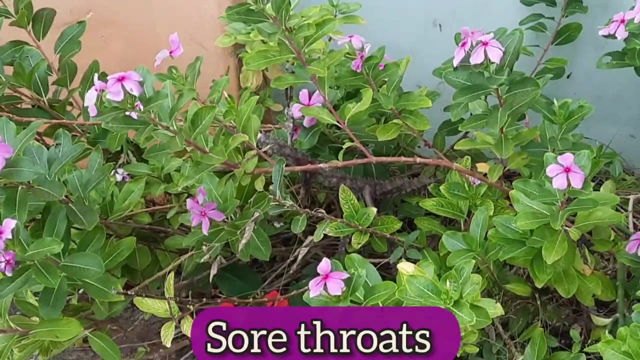 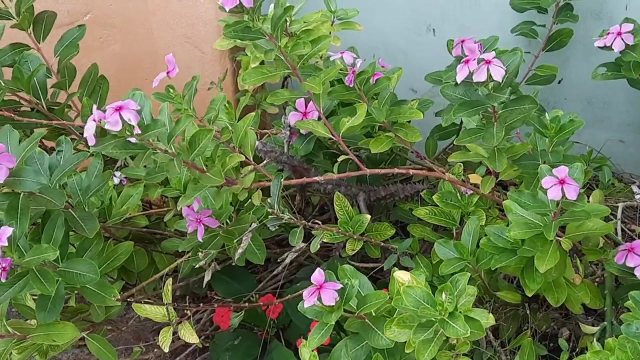 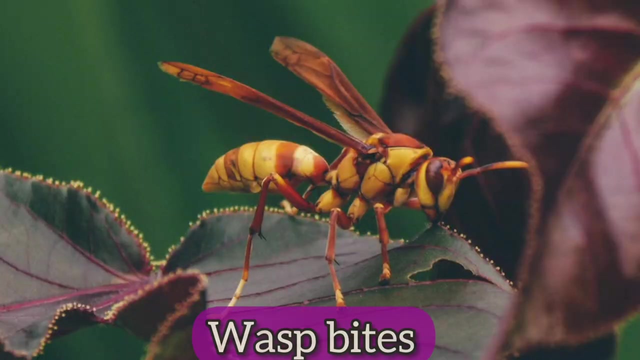 Also to treat colds, coughs and piles. This tea is also used externally to treat sore throats, And they do this by using it as a gargle. People also use the plant externally to treat things like insect bites, you know, like wasp bites or mosquito bites. 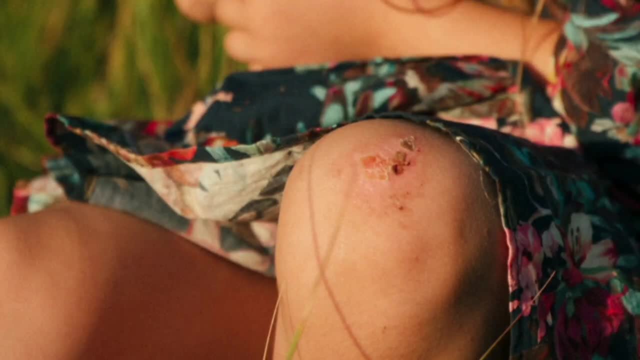 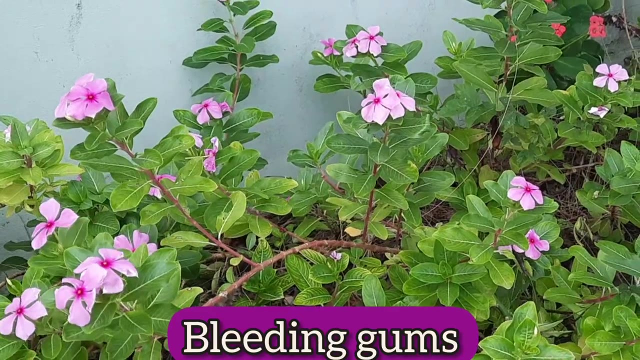 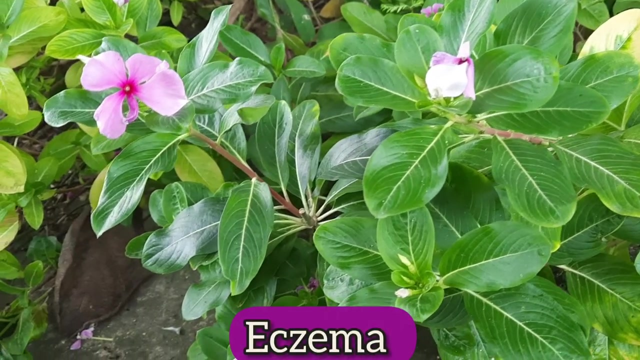 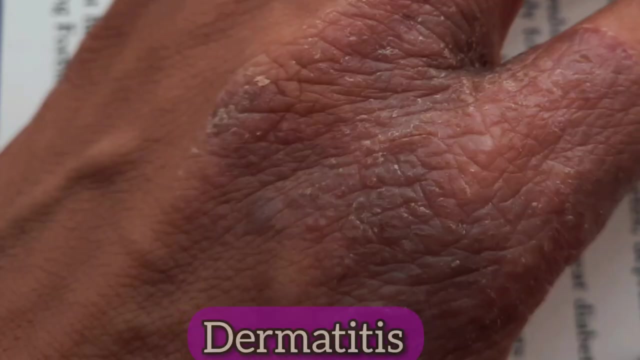 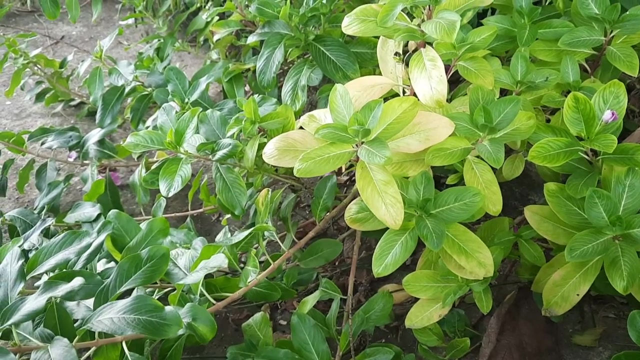 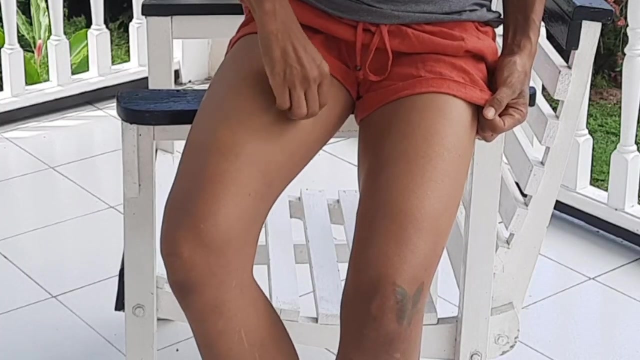 Also to treat insect stings, wounds, canker sores, bleeding gums, nose bleeds and various skin problems, You know, like eczema, acne And dermatitis. One way in which they use the plant to treat these things is to extract the leaf juice and apply it to the affected area. 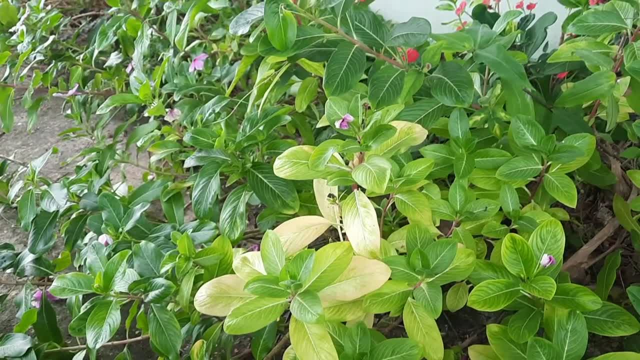 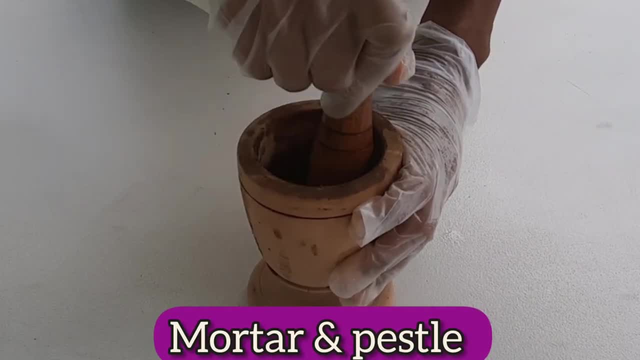 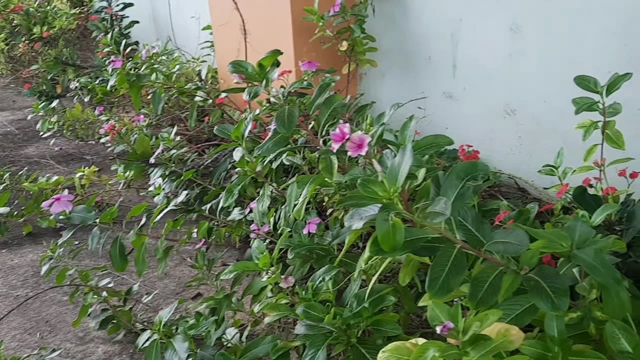 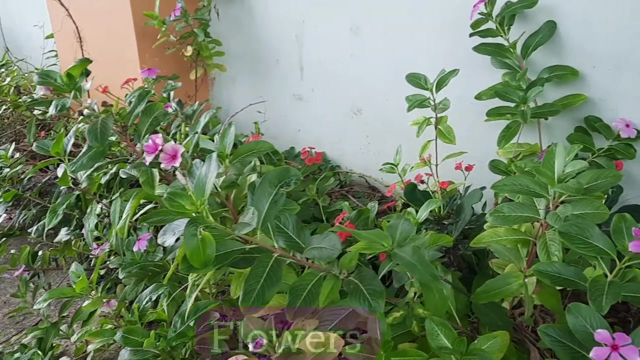 Another way in which they do it is to wash the leaves of the plant and while it is wet, they pound it in a mortar and pestle And then apply the leaves to the affected area For irritated eyes or inflamed eyes. The flowers are used to make tea. 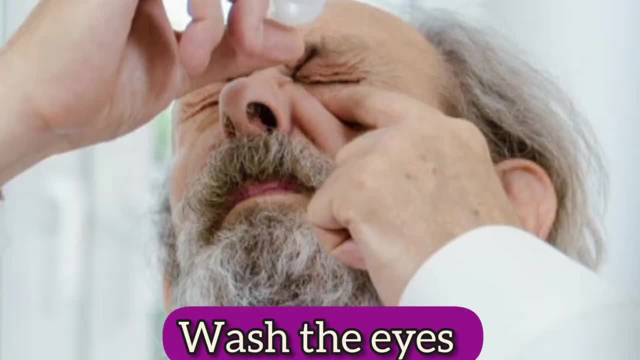 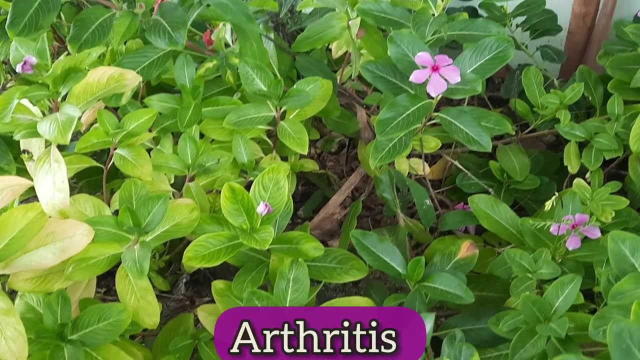 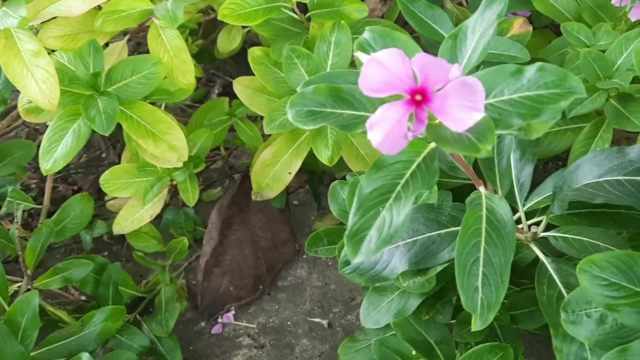 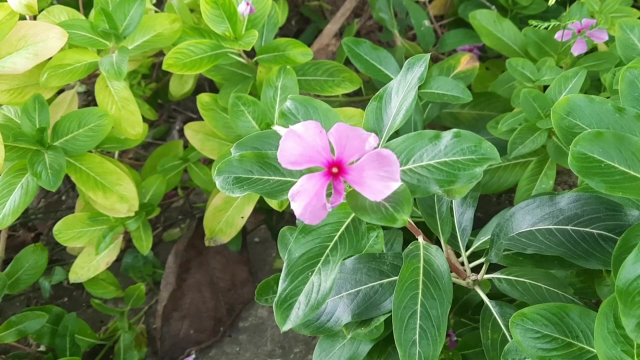 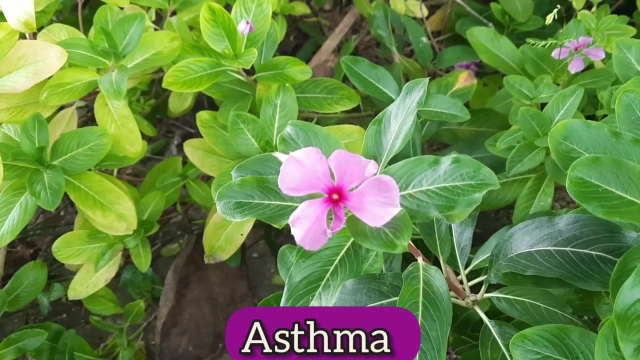 Then it is cooled and used to wash the eyes. Others use the flowers, stems and leaves to treat arthritis and edema And the bruised leaves to topically treat bleeding piles. In Bahamas some people make a tea from the flowers And they take it for flatulence, asthma and tuberculosis. 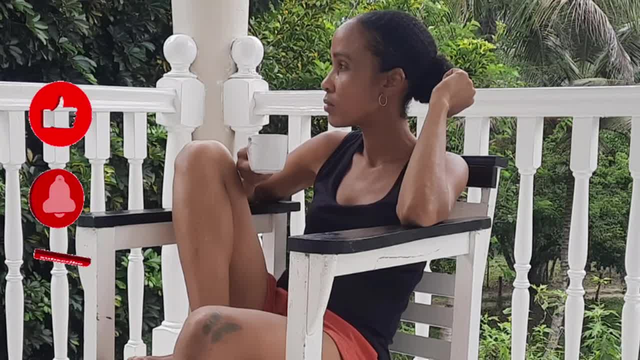 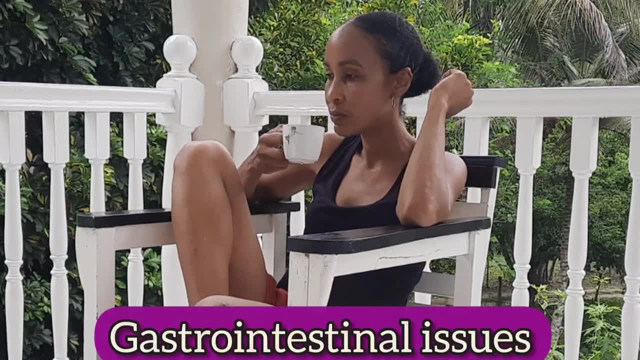 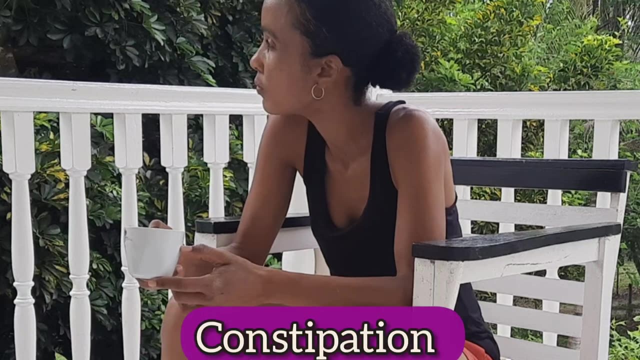 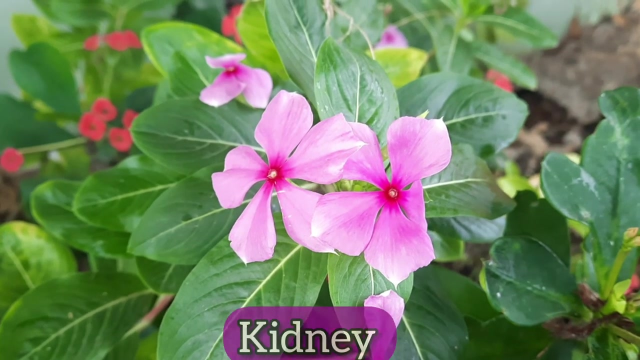 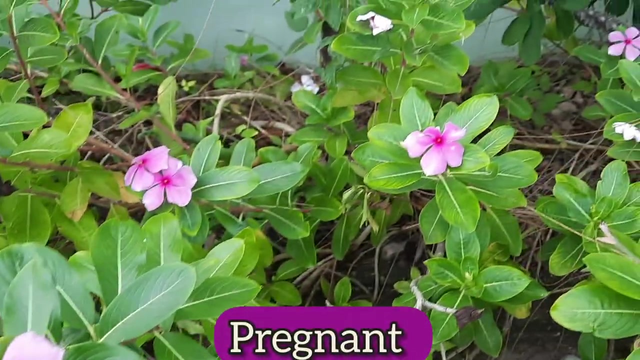 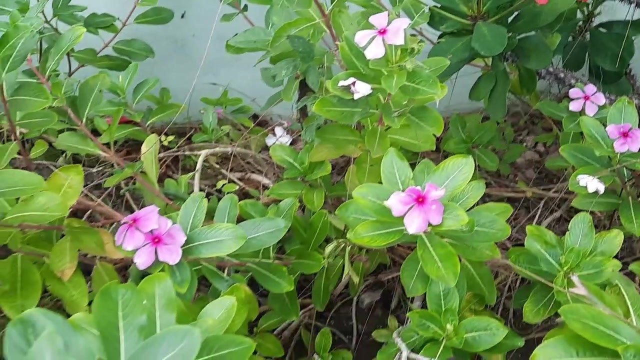 It is said that this tea may cause flushing and gastrointestinal issues, And that you should not drink it if you suffer from constipation, low blood pressure, liver, kidney or lung disease, If you are pregnant or breastfeeding, And before and after surgery.